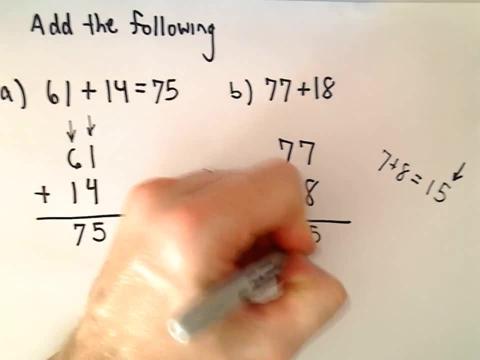 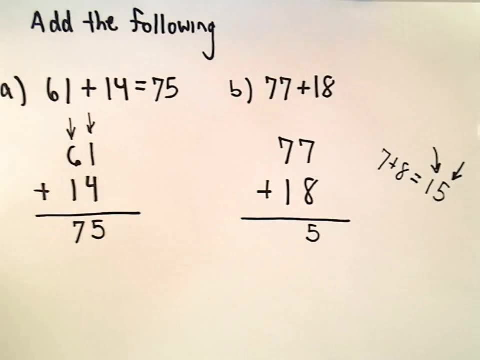 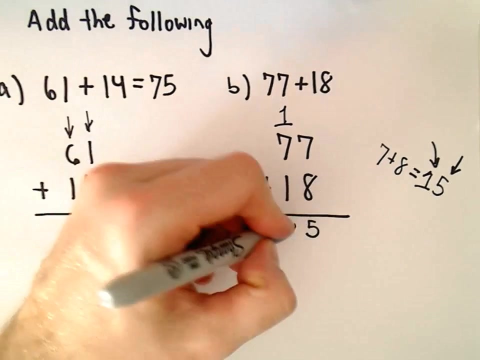 So the 15 is the ones digit. That's the digit we're going to write down. So I'm going to write the ones digit in the ones column. And then our 1 would be our tens digit, so that's what I'm going to carry to the next column. So that 1 is getting carried to the next column. So then I'm just going to add, again, everything in my column. So 1 plus 7 is 8, plus 1 is 9, and it says 77 plus 18, that's going to give us 95. 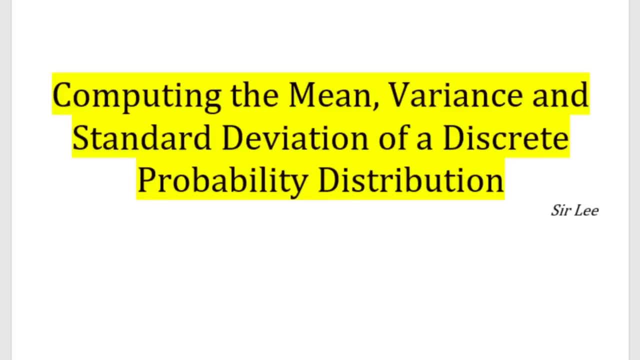 Here is another problem on computing the mean, variance and standard deviation of a discrete probability distribution. Let us have this problem. The number of classmates who are KPAP fans, along with its corresponding probabilities, is given in a table. Compute the mean and the. 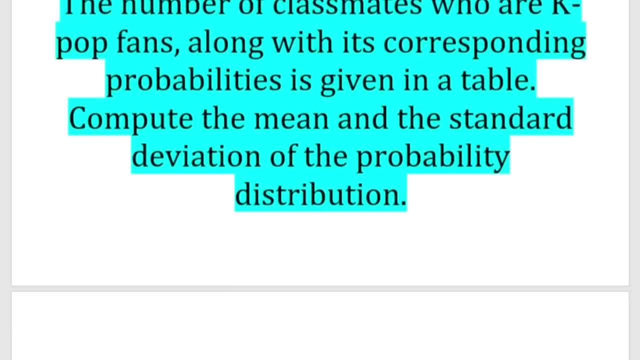 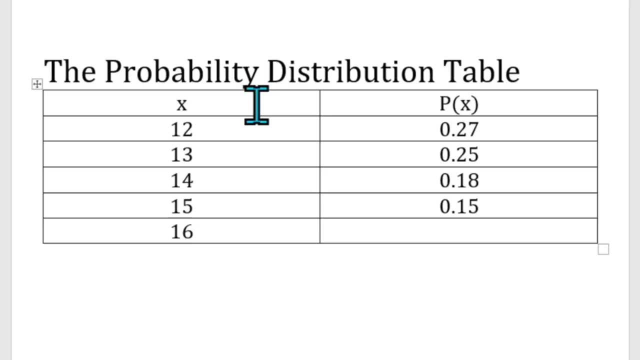 standard deviation of the probability distribution. Here is the given probability distribution table. We have two columns, The first, column x, which refers to the possible values of our random variable, which is the number of KPAP fans, And the second column are its corresponding. 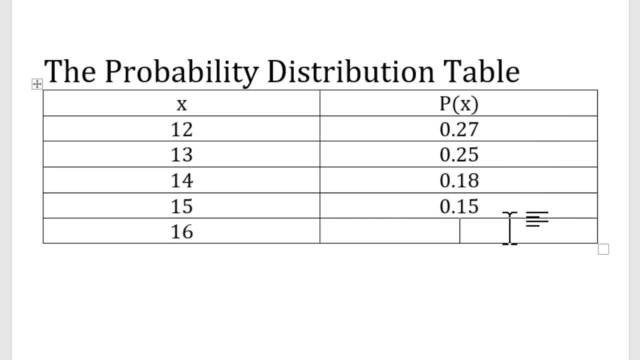 probabilities. If you notice there is a missing probability in this distribution table, Let us always remember that the sum of all these probabilities should be equal to one. In other words, if this occurs, that one or two or one probability is unknown, let us just add. 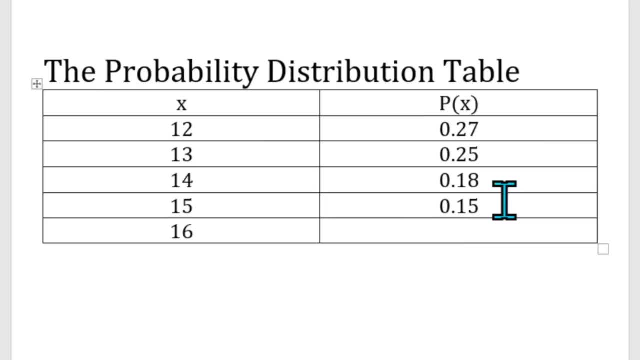 all the given probabilities and subtract the sum from one to get the unknown probability. Let us have: 0.27 plus 0.25 plus 0.18 plus 0.15 is equal to 0.85.. Thus we now found the missing value of the probability in our distribution table. 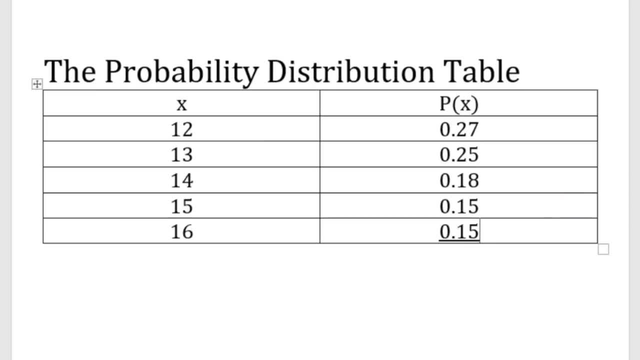 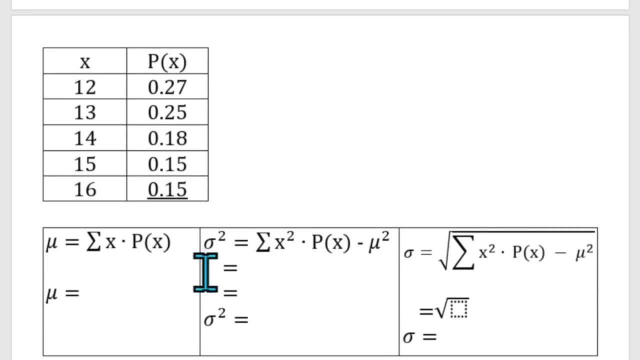 Let us proceed to the process to calculate the means, variance and standard deviation. We have the formula here to solve for the mean. The mean is denoted by mu and it is determined by the binary variance and standard deviation State. the weight of the hard drive, This figure here.